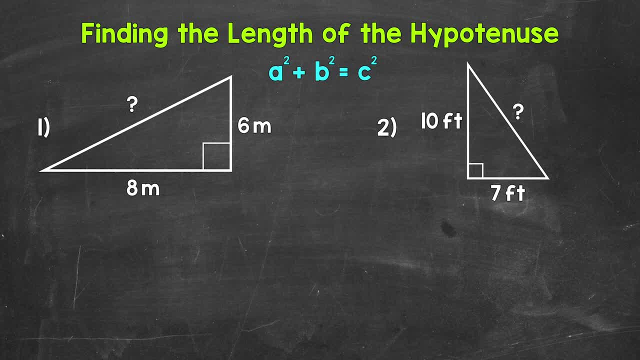 lengths of the legs, The hypotenuse is unknown. Remember, the hypotenuse is the longest side of a right triangle and the side across from or opposite of the right angle. So let's start with the hypotenuse. Let's use a squared plus b squared equals c squared in order to find the length of the 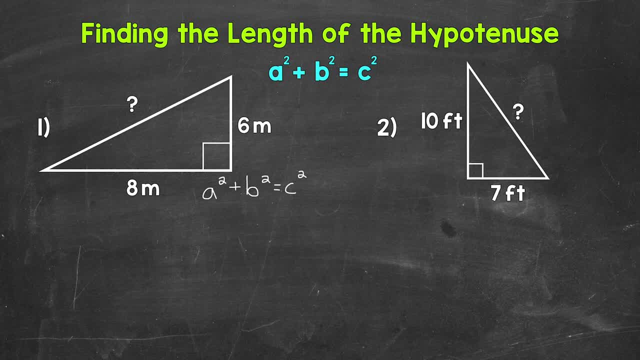 hypotenuse. Now again, c is always the hypotenuse, so this is c, and then the legs are a and b. Let's make this a and this b. Now keep in mind, it does not matter which leg is a and. 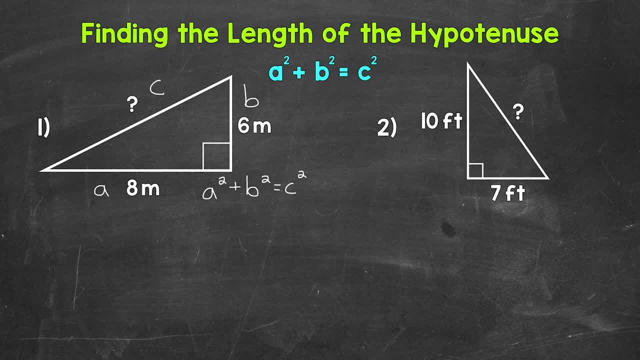 which leg is b. Now we can plug in the side lengths that we are given and work through the equation in order to find the length of the hypotenuse. So a is 8 meters, so let's plug in 8 for a. so 8 squared plus b is 6 meters, so plug in 6 for b, so 6 squared equals c squared. 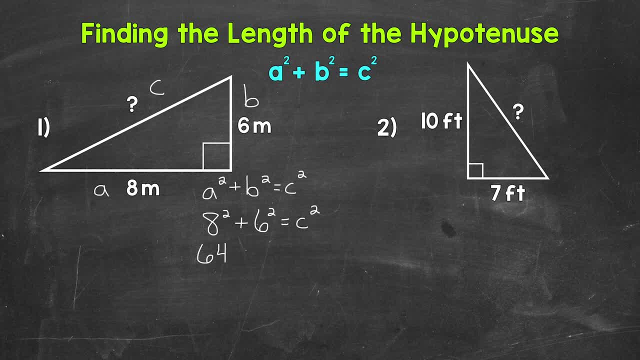 8 squared. 6 squared gives us 64, plus 6 squared gives us 36.. 64 plus 36 is 100, so 100 equals c squared. Our next step is to isolate c in order to figure out what c equals. So again, we are just working. 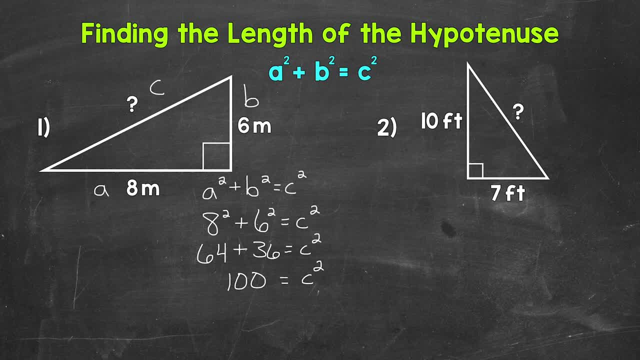 through this equation to figure out c. Since c is being squared, let's take the square root in order to isolate c. Whatever we do to one side of the equation, we must do to the other, so we need the square root of 100 as well. 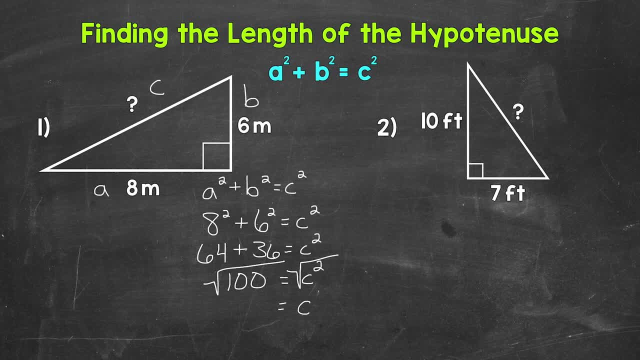 c is now isolated, so we have c equals, and then the square root of 100 is 10,, so c equals 10.. Let's rewrite that with c squared, So c equals 10, and this is meters. So the hypotenuse measures 10 meters, and that's our missing side length. 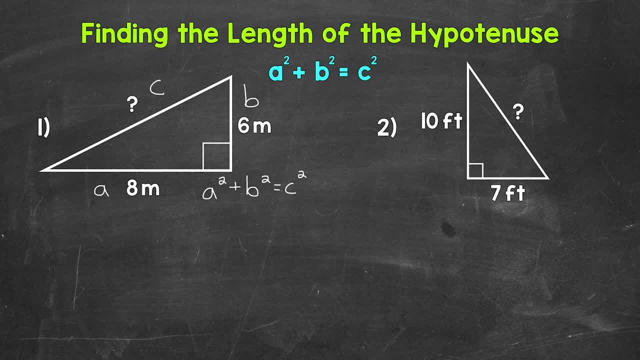 which leg is b. Now we can plug in the side lengths that we are given and work through the equation in order to find the length of the hypotenuse. So a is 8 meters, so let's plug in 8 for a. so 8 squared plus b is 6 meters, so plug in 6 for b, so 6 squared equals c squared. 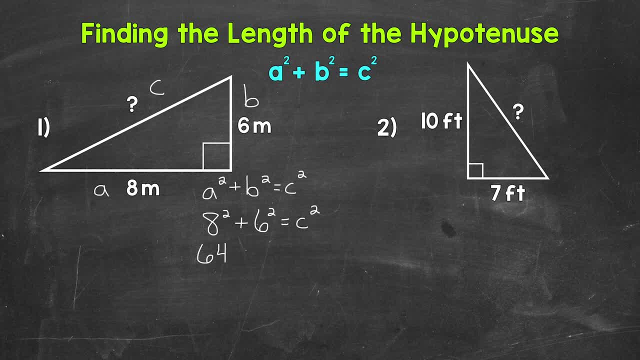 8 squared. 6 squared gives us 64, plus 6 squared gives us 36.. 64 plus 36 is 100, so 100 equals c squared. Our next step is to isolate c in order to figure out what c equals. So again, we are just working. 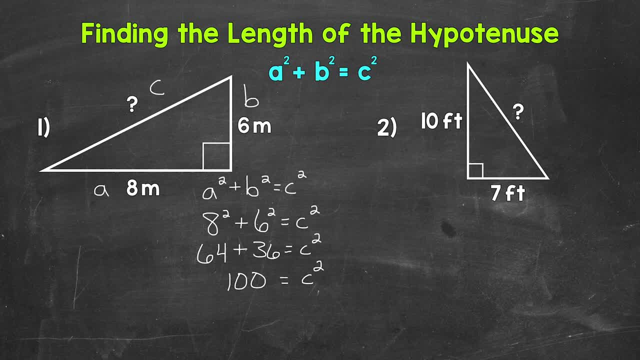 through this equation to figure out c. Since c is being squared, let's take the square root in order to isolate c. Whatever we do to one side of the equation, we must do to the other, so we need the square root of 100 as well. 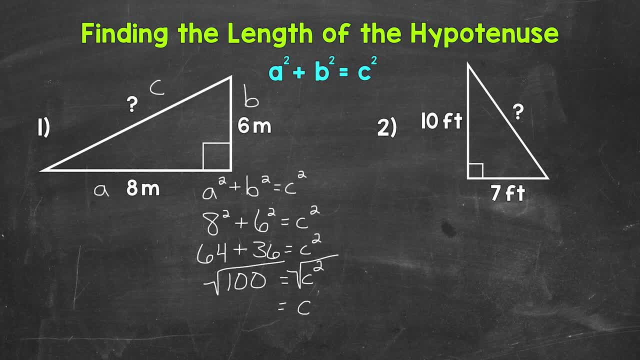 c is now isolated, so we have c equals. and then the square root of 100 is 10,, so c equals 10.. Let's rewrite that with c, So c equals 10, and this is meters, So the hypotenuse measures 10 meters, and that's our missing side length. 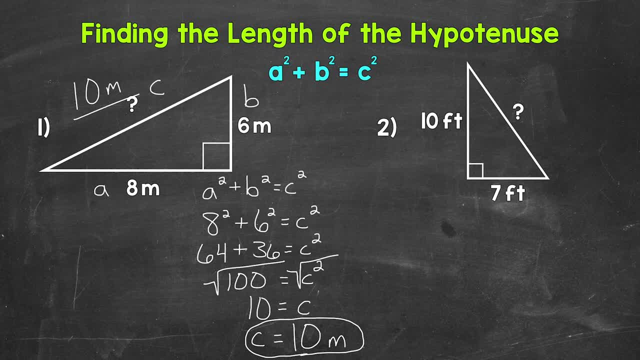 Let's move on to number two, where we have a right triangle and again we need to find the length of the hypotenuse We are given the two legs. We have 10 feet and 7 feet, so let's use a square root. 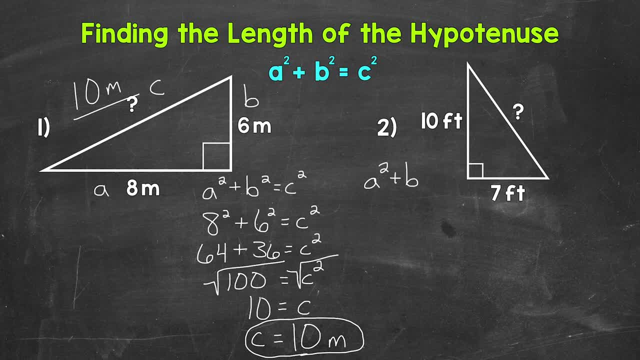 Let's call this leg a, this leg b, and then the hypotenuse is c. Now we can plug in and work through this equation. So for a we have 10 feet, plug in 10 for a, so 10 squared plus 7 feet for b, so that gives us 10.. 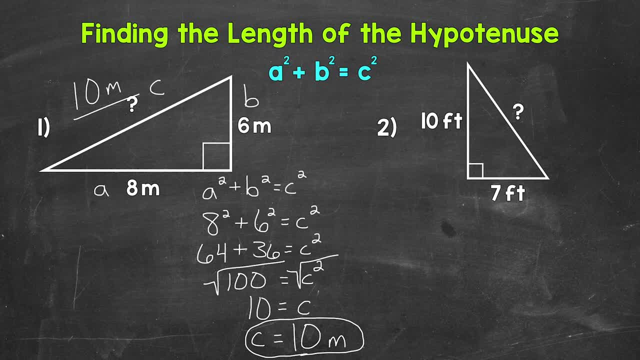 Let's move on to number two, where we have a right triangle and again we need to find the length of the hypotenuse We are given the two legs. We have 10 feet and 7 feet, so let's use a square root. 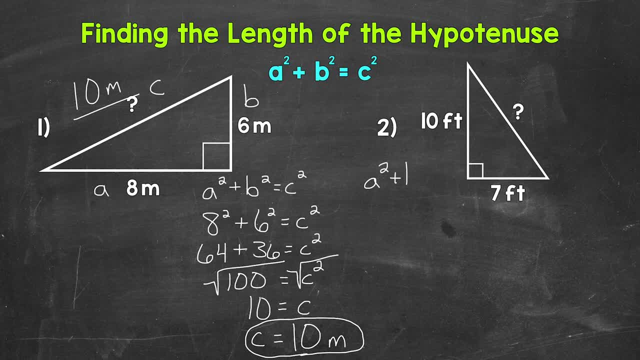 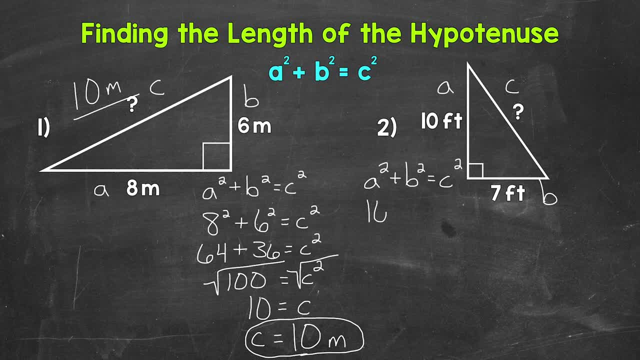 so for a we have 10 feet, plug in 10 for a, so 10 squared plus 7 feet for b, so plug in 7 for b. 7 squared equals c squared. 10 squared that's 100, plus 7 squared that's 49. 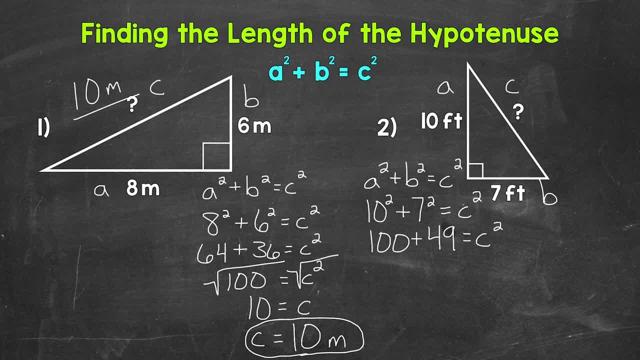 equals c squared. 100 plus 49. that gives us 100 plus 49. that gives us 149 equals c squared. now we have 149 equals c squared. so our next step as we work through this equation, is to isolate c. c is being squared, so let's take the square root in order to isolate c. 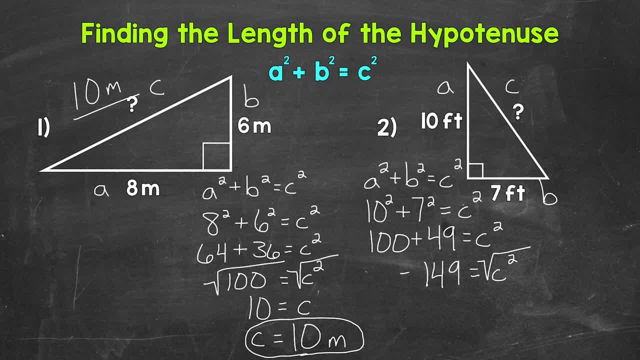 whatever we do to one side of the equation, we must do to the other. so let's take the square root of 149 as well. we end up with an isolated c on the right side of the equation, and then, as far as the square root of 149, 149 is not a perfect square, so we do not end up with 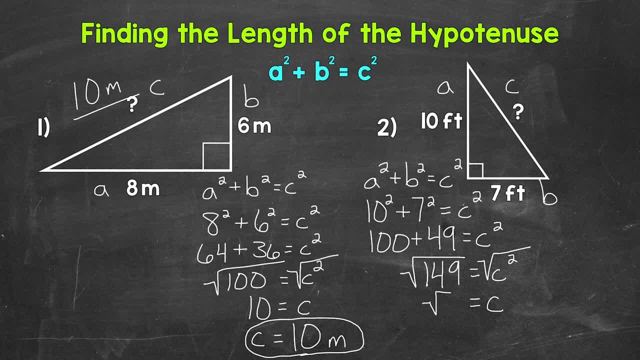 a whole number. answer c equals the square root of 149. now we can write the square root of 149 as an approximate rounded decimal. the square root of 149, 149 is irrational, The decimal never stops and it doesn't repeat. So again, let's round it and we. 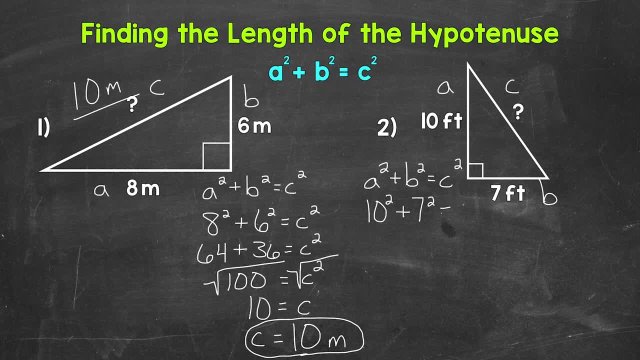 And then we have a right triangle and again we need to find the length of the hypotenuse. Let's use a square root, so 10 feet, and then the hypotenuse is c. So plug in 7 for b. 7 squared equals c squared, 10 squared, that's 100 plus 7 squared, that's 49. 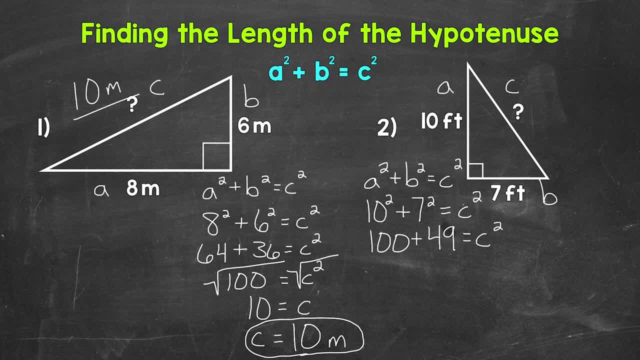 equals c squared. 100 plus 49, that gives us 149 equals c squared. Now we have 149 equals c squared. So our next step as we work through this equation is to isolate c. c is being squared, So let's take 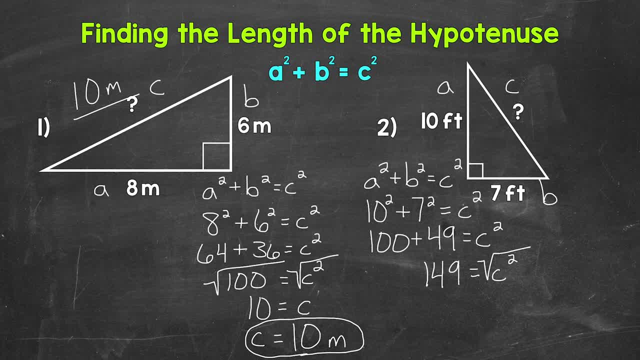 the square root in order to isolate c. Whatever we do to one side of the equation, we must do to the other. So let's take the square root of 149 as well. We end up with an isolated c on the right side of the equation, And then as far as the square root, 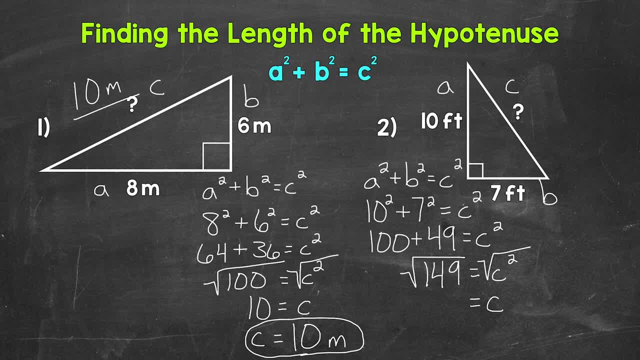 of 149,. 149 is not a perfect square, So we do not end up with a whole number. answer: c equals the square root of 149.. Now we can write the square root of 149 as an approximate rounded decimal. The square root of 149 is irrational. The decimal never stops and it. 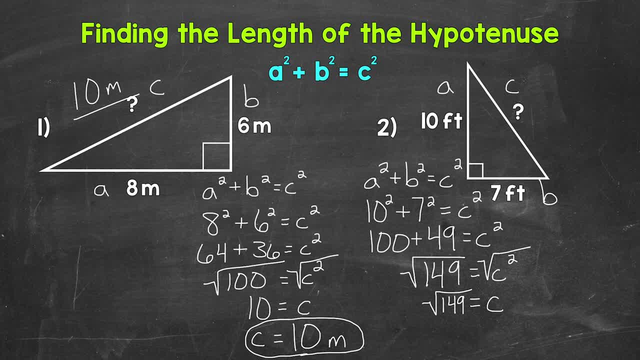 doesn't repeat. So again, let's round it, and we will round it to this. So the square root of 149 gives us 12.206. and again that just continues on. So I'm going to write it to the thousandths place and then round it to the hundredths. So let's round it to the. 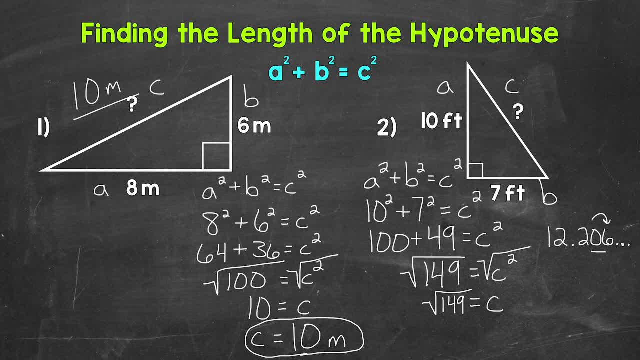 hundredths place We have a 6 to the right in the thousandths. So this rounds up. So the square root of 149 is irrational. The square root of 149 is irrational. The decimal never stops and it doesn't repeat. So the square root of 149 is approximately 12 and 21 hundredths. So c is approximately 12 and 21 hundredths and this is feet.